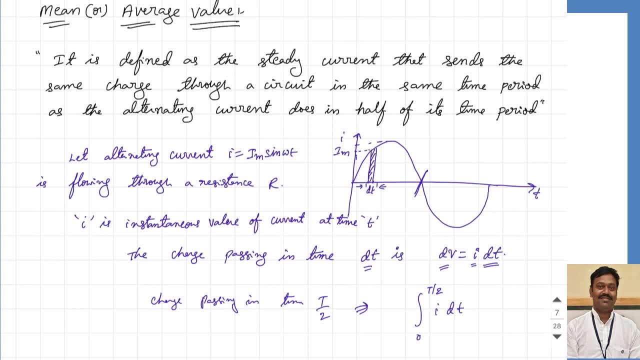 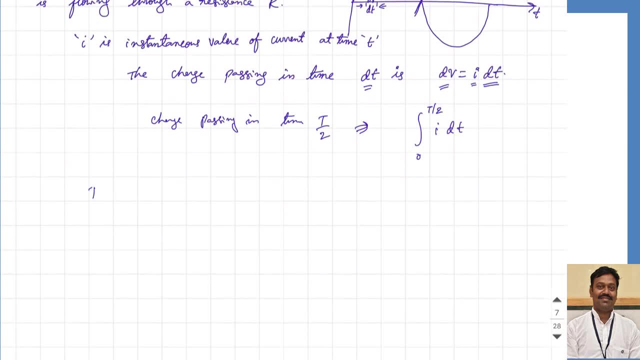 integration of that I dt. we have to do the integration from 0 to t by t. So let us assume this average value of the current. that average value of the current is represented by I average. Let this be the average value of the equal and dc current, or it is a equal and dc current. 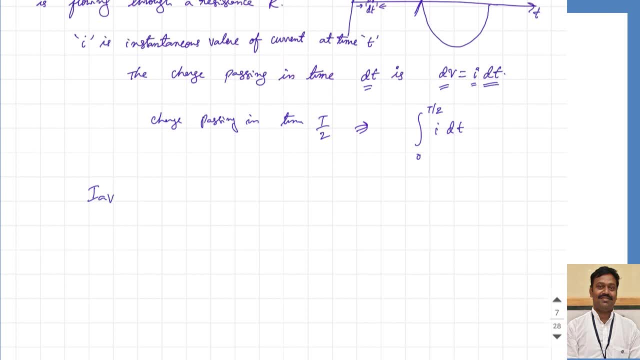 that transfers the same amount of charge. so that is represented by i average, or this is also called as mean value of the current. so if this mean value of current is passing for time t by 2, because both should be same- then the total charge transferred will be equal to that i average value. because in the case 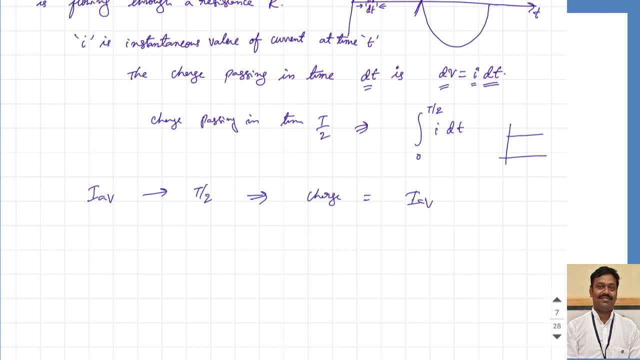 of dc. we know the value is constant so i have to simply multiply the current with the time period so i can multiply. i average into the time period will give my total value of the charge that is transferred. so as per this average value definition, so this should be equal to the 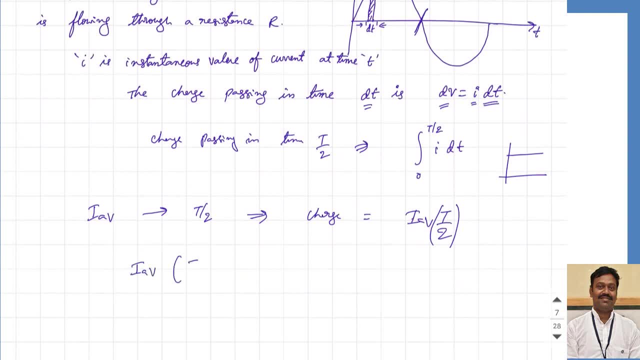 integration. so i can tell that this i average multiplied by t by 2 should be equal to integration from 0 to t by 2 into idt. so i am just substituting the value of i, so we know that the value of i, instantaneous value, is nothing but i maximum sine omega t into dt, or from this i can write my value. 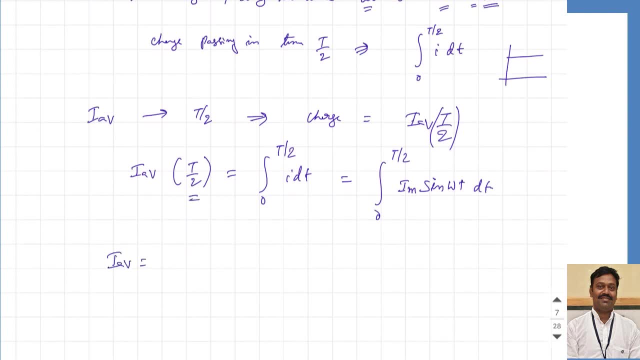 i average value will be equal to this t by 2. i can bring to the second side, so this becomes 2 by t integration from 0 to t by 2: i maximum sine omega t. i maximum sine omega t dt. so if you do this, 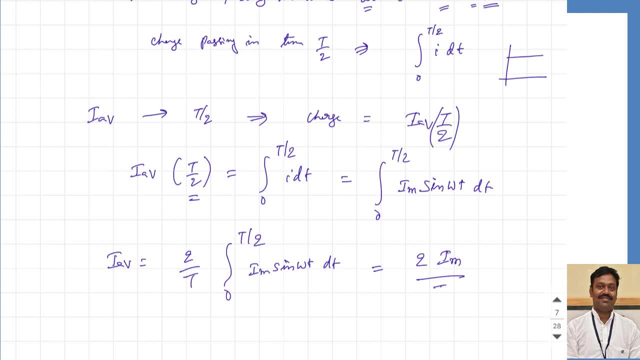 integration. this becomes 2 times of i maximum by t, because i maximum is constant, so d by dt. so the integration of sine omega t is minus cos omega t divided by omega. integration is from 0 to t by 2. integration is from 0 to t by 2. if you substitute this, you will: 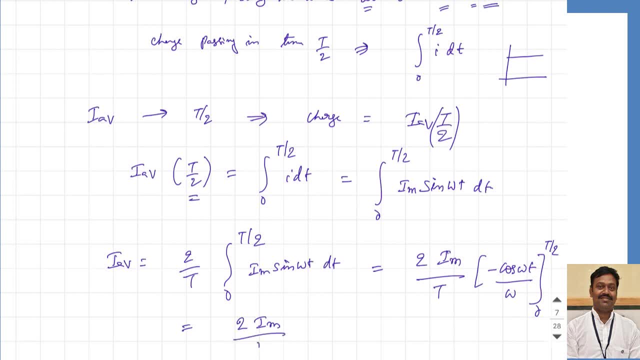 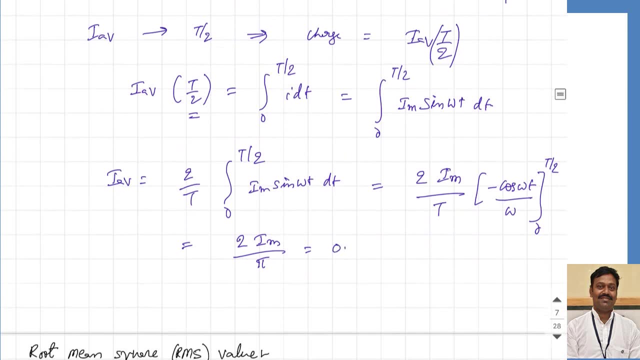 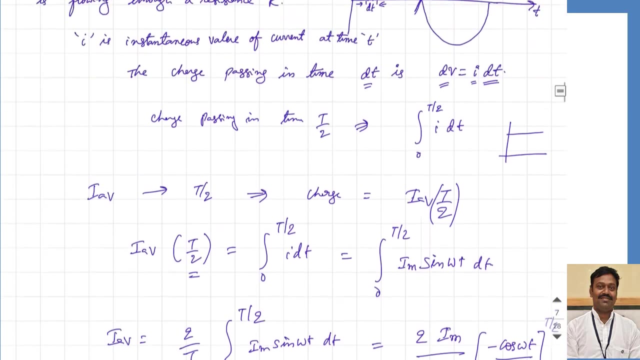 get this as 2 times of i maximum by pi. you can just substitute it and calculate it. you will get it at 2 times of i maximum by pi, or this will be equal to 0.637 times of i maximum. this is for the case of sinusoidal wave. so here one thing you have to remember whenever you are calculating the. 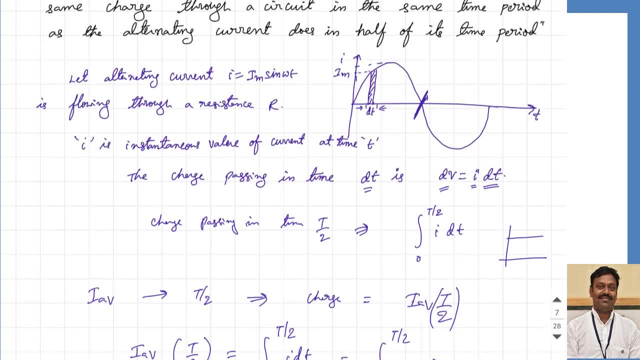 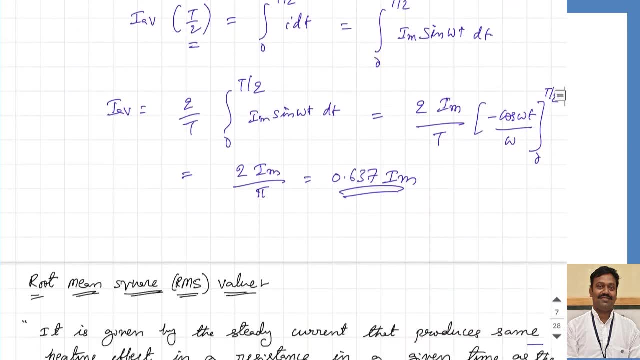 average value. if the waveform is symmetrical, then you have to take for half cycle. if waveform is not symmetrical, then you have to take the integration for full cycle. let us take the example. so let us take, for example, the output of a full wave rectifier. we are going to see in analog 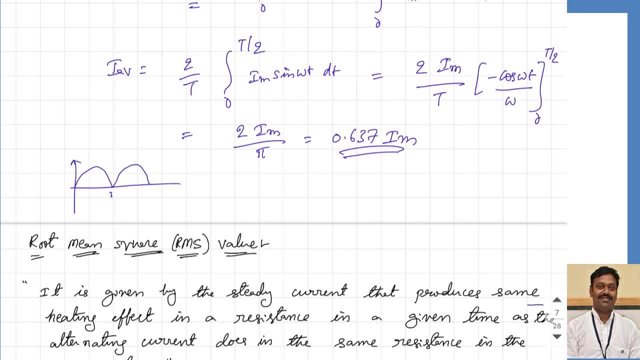 electronics. the output of a full wave rectifier will be like this: that means pi and 2 pi. so you can see here this is symmetrical about this. so in this case you have to do the integration from 0 to pi only. 0 to pi only. there may be another case: half wave rectifier. half wave rectifier means: 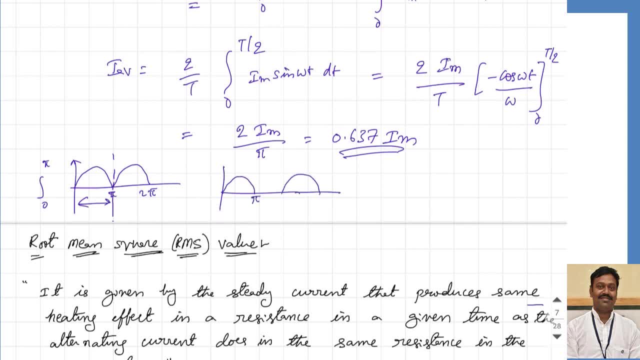 only half of the wave will come. that means it will conduct from 0 to pi and pi to 2 pi. it will not conduct. so in this case you have to do the integration from 0 to 2 pi because it is symmetrical about this. that means up to here. 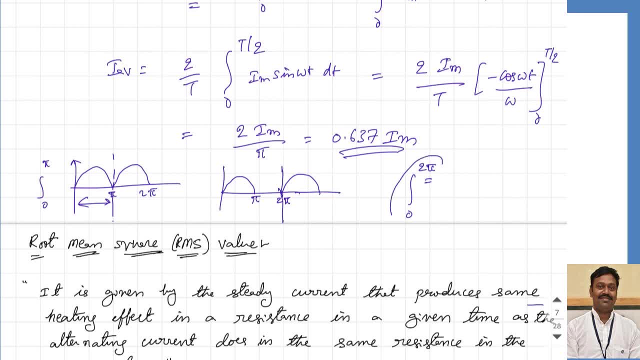 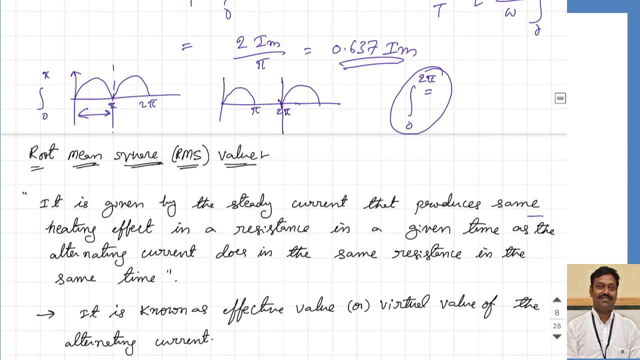 it is one wave, again it is repeating. so that's why you have to do the integration from 0 to 2 pi. anyway, the details of these things, how to analyze, we are going to solve the numericals after discussing all these basics. i will discuss in detail there. so now coming to the next one. 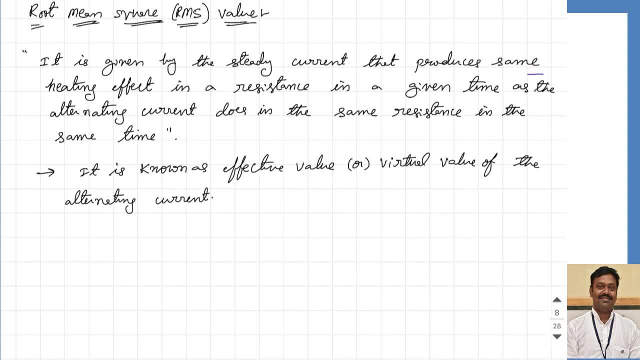 root mean square value. the average value is dealing with the charge transfer. now root mean square value will deal with the energy transfer. so it is given as the steady current that produces same heating effect in a resistance in a given time as the alternating current does in the same. 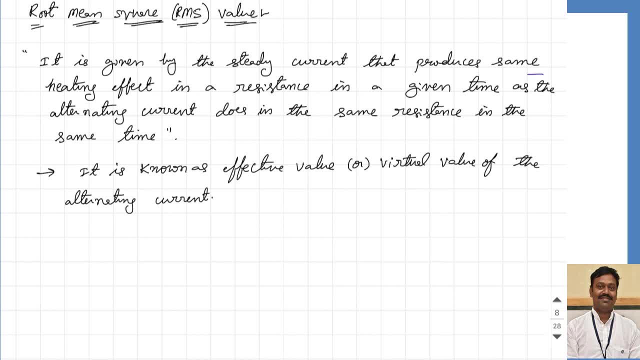 resistance. in the same time, that means we are correlating the heat that is produced. so that's why this is also called as the effective value, because the major purpose of electrical power is to transfer the energy or to produce the heat that is produced. so that's why this is also called as the effective value, because the major 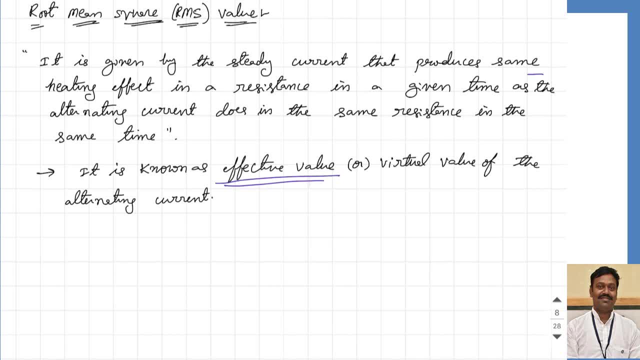 in the initials ages, when it is first invented. the incandescent lamp also based on the principle of heat, and mainly it is used for the heating purpose in the homes. so that's why this represents what is the effective value- or this is also called as a virtual value- of the alternating current. 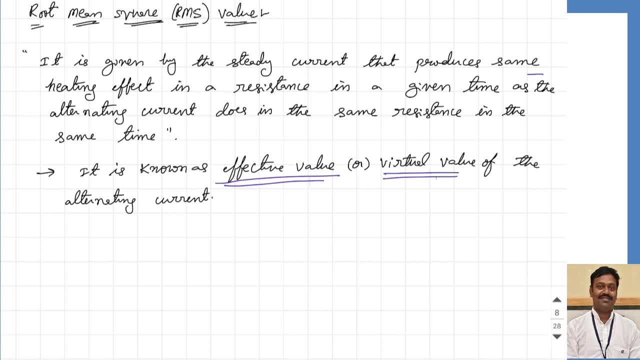 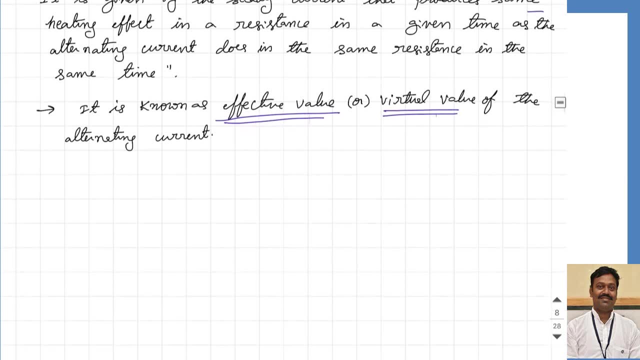 because alternating current is continuously changing. we are representing what is the equivalent value compared to the dc to produce the same value of the heat, because initially dc is invented, then ac came. we have seen in the basics, so now how to calculate this. so again same thing. i am assuming that the heat produced. 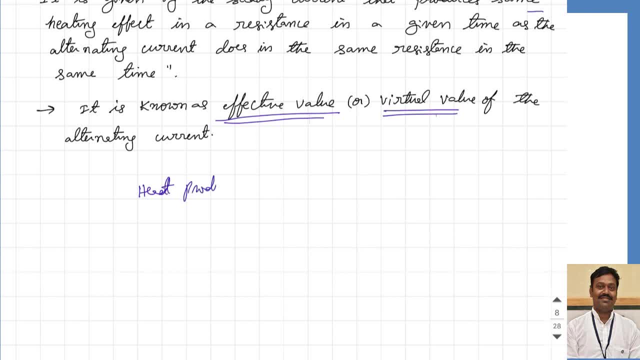 heat produced in time dt will be equal to. let us take it as h. i am taking dh, the small change, because we know heat is equal to i square r loss, so i square r into dt, you agree with me? so now the heat produced in time t by 2. so heat produced in time t by 2 will be equal to the heat produced in. 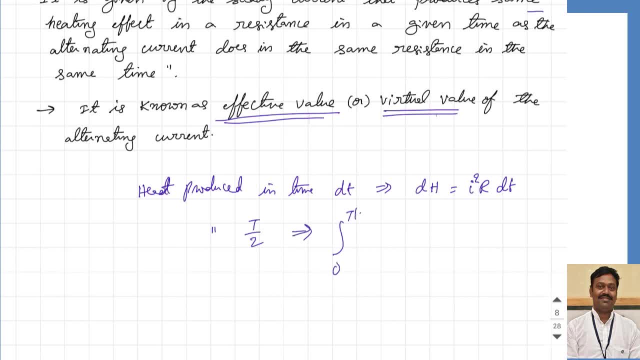 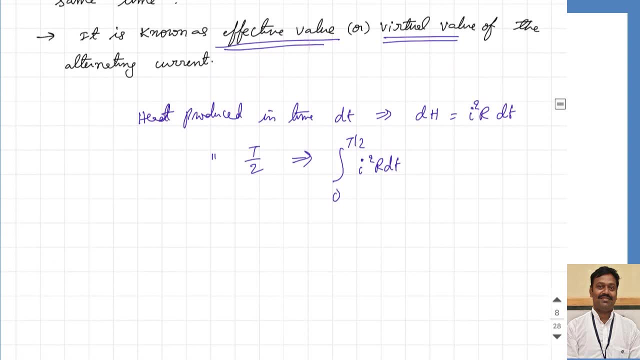 time t by 2, so i have to take i square into r, into dt. so let us assume the rms value that can produce this. i am representing by the value i rms. this represents the a colon dc value which can produce the same heat. so in this time what will be the heat produced? the heat produced will be equal. 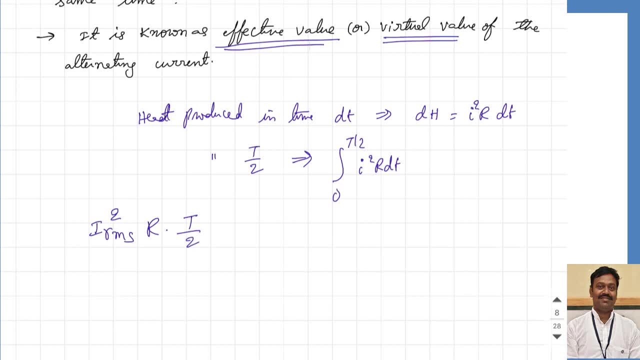 to i square r multiplied by the time, the time period we are taking- is t by 2. so a colon dc heat that will be produced will be irms. square into r, into t by 2. this will be equal to this integration: 0 to t by 2. so i square, so we know i is equal to i maximum sine omega t whole square into r, into dt. 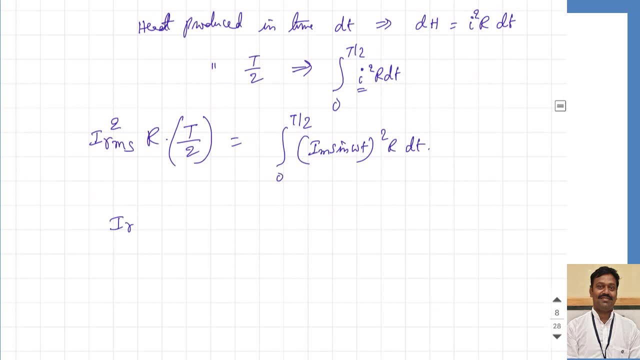 this is what we can write. so from this i can write: irms square is equal to. because r is same in both sides, because it is constant. i can cancel it out. so this becomes 2 times of i maximum by t and i maximum is actually i maximum square. this become i maximum square sine square, omega t. 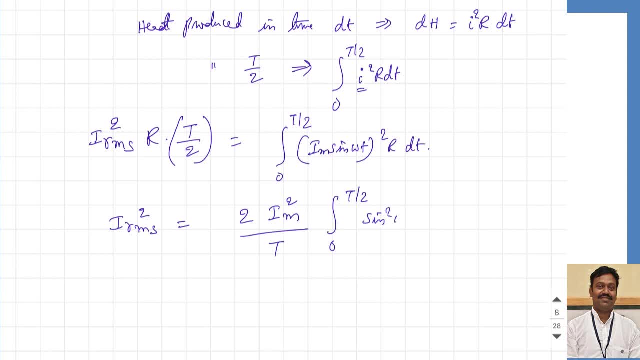 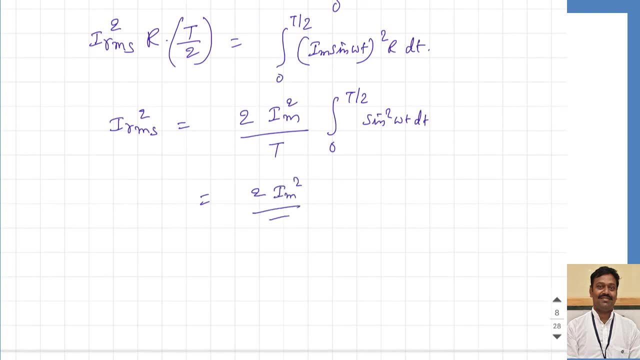 so this becomes integration from 0 to t by 2 sine square omega t, dt. or this i can write as 2 i maximum square divided by t. so sine square omega t, i can write as 1 minus cos 2 omega t divided by 2 into dt. so this 2 and 2 will cancel. 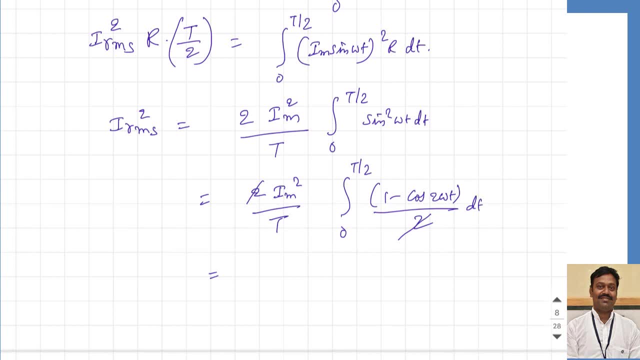 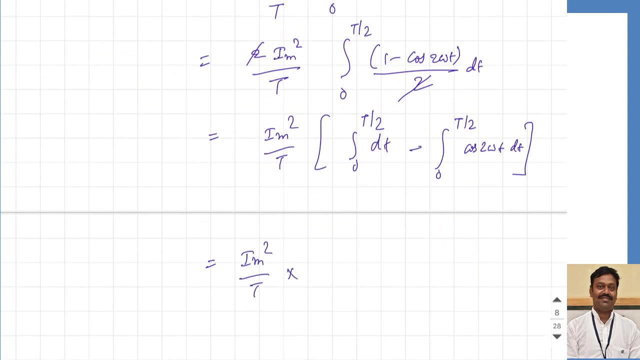 so if you substitute the values and expand this so you will get this as i maximum square divided by t, integration from 0 to t by 2 dt first term, minus integration from 0 to t by 2 cos 2 omega t dt. you got this. so then this will be equal to i maximum square by t into if you substitute it. 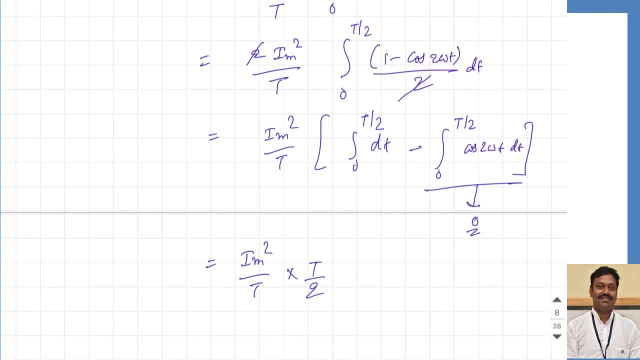 you will get it as t by 2, because this integration, this term, will become equal to 0. you can just substitute and cross verify the integration from 0 to t by 2. cos 2, omega t, dt will be equal to 0. so we get it as i maximum square. this tt will cancel. this becomes i maximum square. 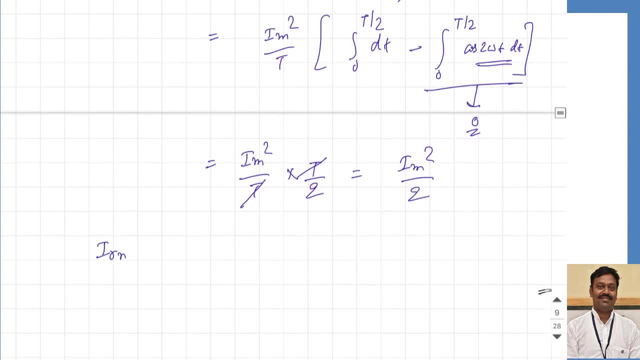 divided by 2. so i am writing the value. what we get: irms square is equal to i maximum square by 2. so from this i can calculate my rms value. rms value will be equal to i maximum by root 2. this is the rms value for the alternating quantity. 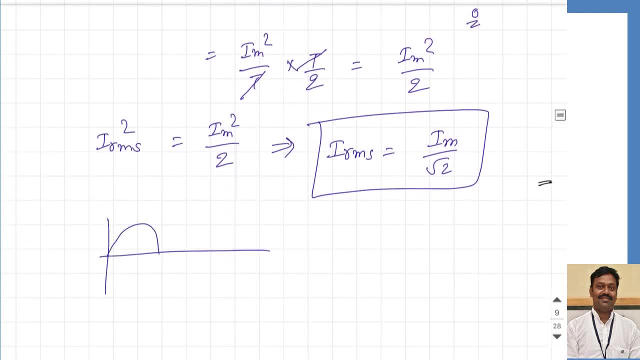 so same rms value you will get for the case of fully rectified sine wave also because it is symmetrical. again, i can take the rms value for half cycle only, so it will give the same value. but if you are taking for the halfway rectified wave, 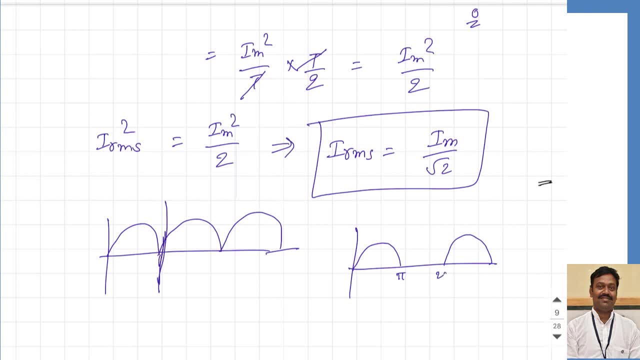 halfway rectified wave you can see only up to pi. it will produce heat. from pi to 2 pi, the current is equal to 0. it will not produce any heat. so you have to take the rms value for this whole cycle. accordingly, your rms value will decrease for the case of half wave, rectified sine wave. 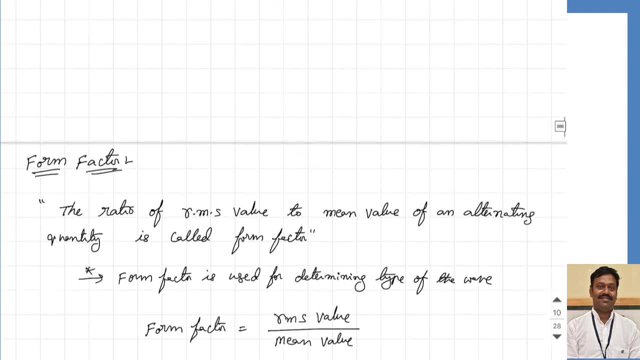 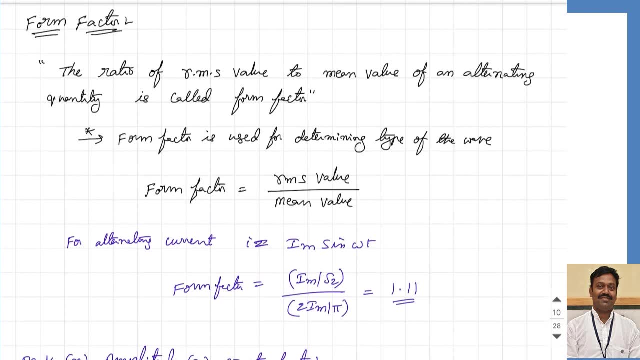 so you have to remember this. so now let us proceed further. so next one, i am going to see form factor. form factor is the ratio of rms value to the mean value of the alternating quantity. it is a ratio of rms value divided by mean value. what does this indicates? the form factor is used in determining. 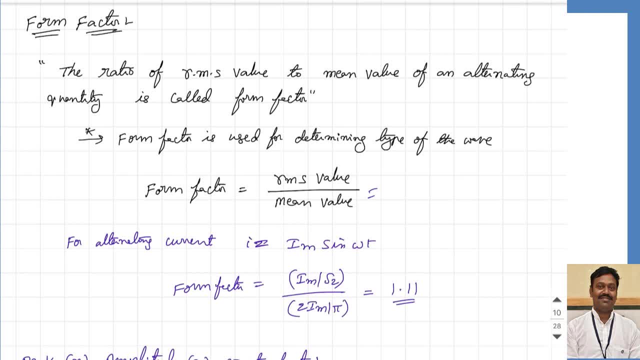 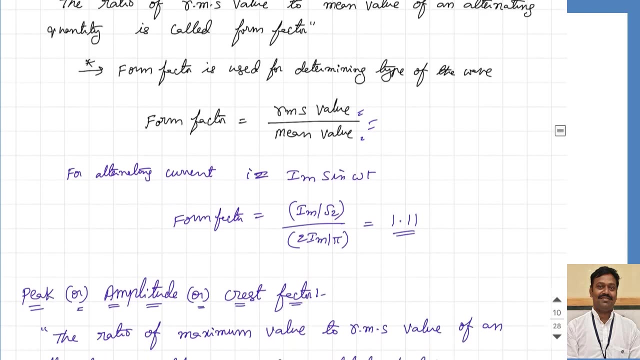 what is the type of the wave, because different waves will have the different rms value on the mean value and that ratio will be different for different type of signals. so we can know easily what is the type of the signal that is passing through this using the form factor, like, for example, if you take the alternating current or a full. 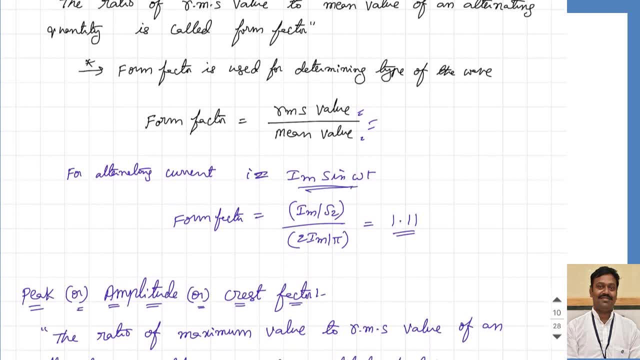 wave rectified output where the current is given by i max 1, sine omega t form factor will be equal to rms value is i maximum by root 2 and average value is 2 times of i maximum by 5 that we have already derived will be equal to 1.11. it will not be same for other waveforms. you can check it for. 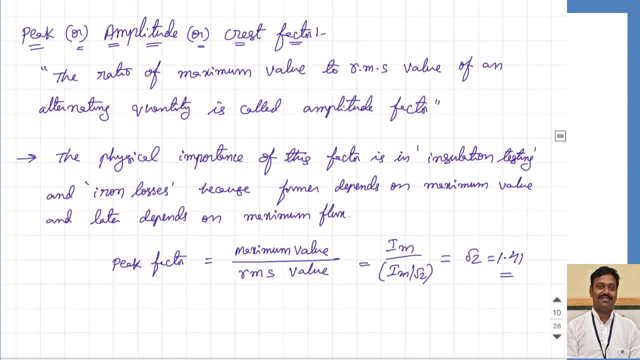 other waveforms. we are going to derive some numericals there. i will discuss this again. then there is another factor called as peak or amplitude or crest factor. so what is the name of this? this is the ratio of maximum value to the rms value of an alternating quantity. that means 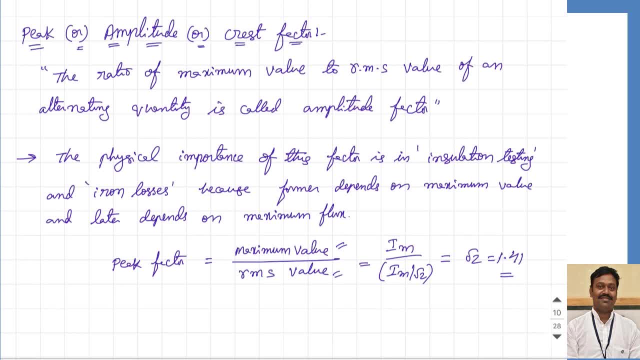 this peak factor is a ratio of maximum value by rms value. if you substitute for the normal sinusoidal wave, you will get it as 1.41. so what does it signify? the physical importance of this factor is in insulation testing and iron losses. so what does it mean? so the insulation strength of any material so will depend on the dielectric. 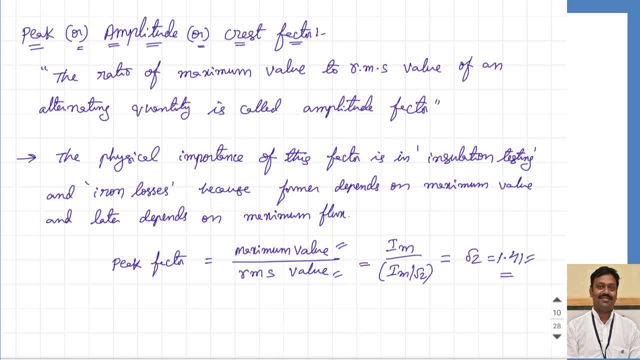 strength. you have studied in electromagnetics that the dielectric strength will depend on what is the peak value of the voltage across applied across its two sides of the material. that means whenever you want to test the insulation of any material, that insulation capacity of the material will depend on the peak value of the applied voltage. similarly, if you take 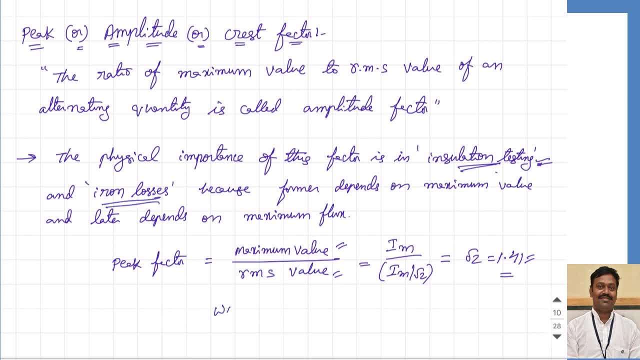 the iron losses. that iron losses, there are two types. one is hysteresis loss and second one is eddy current loss. hysteresis loss depends on b maximum to the power of 1.6 and eddy current depends on b maximum square. this is the maximum value of flux density. 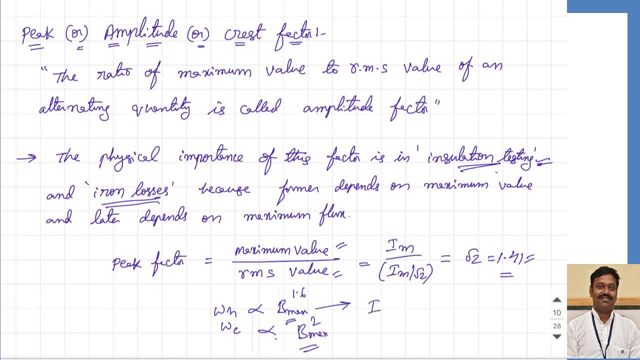 again this maximum value of flux density. flux density is produced because of current, magnetizing current, and this current is produced because of your applied voltage. that means the maximum value means it will depend on ie maximum, this depends on v maximum, so this is in turn again depending on the peak value. that's why 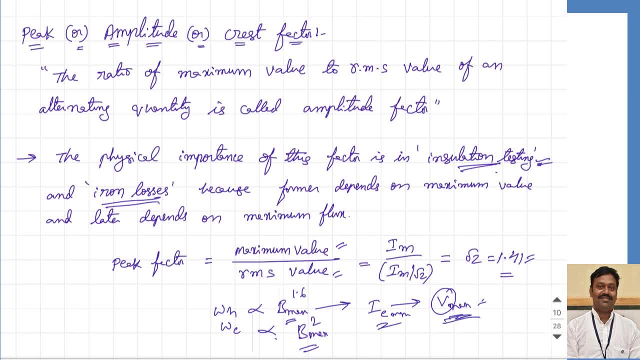 this factor will be useful to know the maximum value. what is the ratio? so we know the rms value. like, for example. always the rating of electrical equipment is given in rms values one way. like, for example, your supply voltage is 230 volts, that means it is not peak value, it is the rms value. 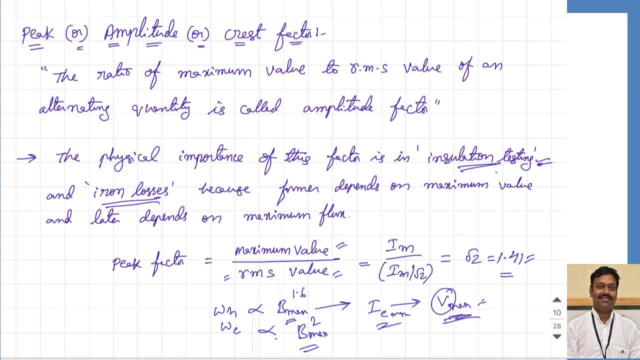 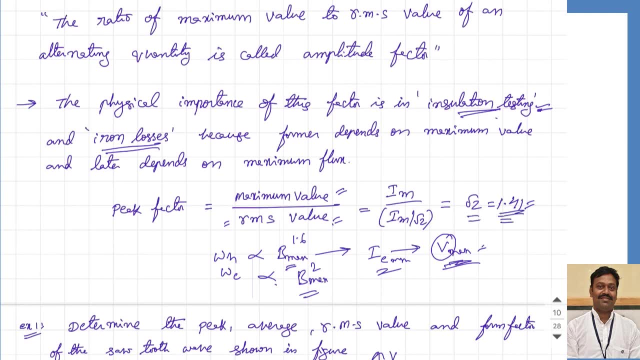 is 230 volts. if you want to calculate the peak value you have to multiply with root 2. so in that case we can divide the maximum value divided by rms value how much you will get root 2. that means in a normal sine wave this ratio is 1.41. so for example, some other wave is there that is given. 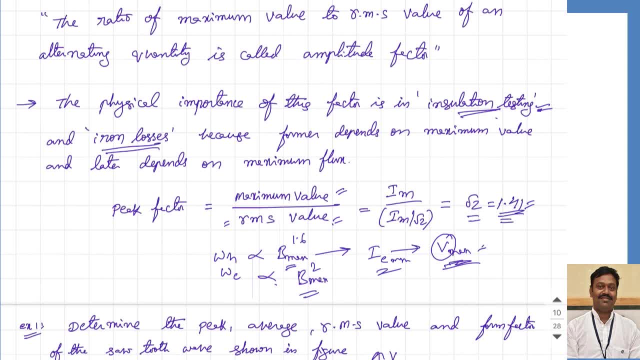 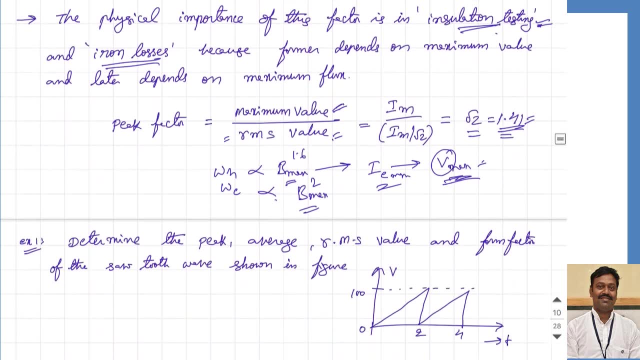 always the rating is given in rms. how will i know my insulation strength? i can know by knowing what is the actual maximum value of that particular wave, because out of all the waves, sine wave is the most efficient one. so let us try to solve some numericals to clarify whatever we have discussed. 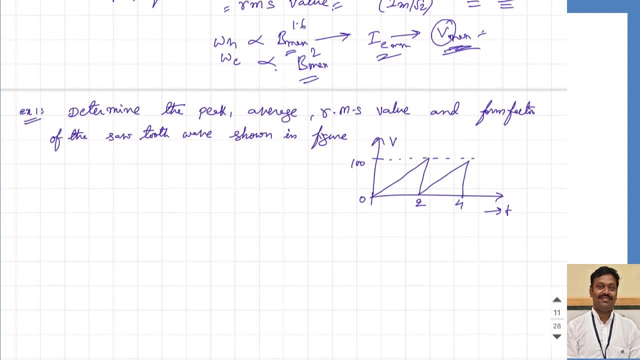 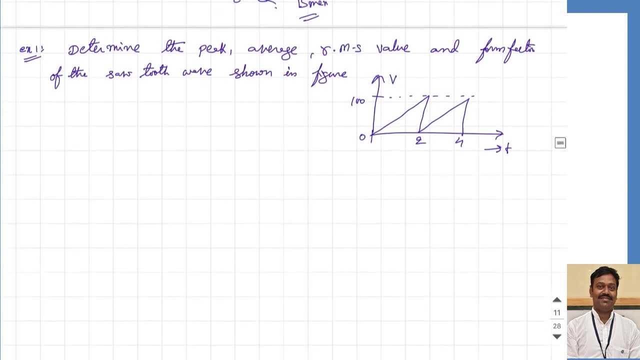 till now. so example number one: determine the peak average rms value and form factor of a sawtooth wave shown in the chart, the figure. it is a sawtooth wave. so first thing, whenever anything is given, you have to write the equation for this waveform. so you can write the equation for this waveform. 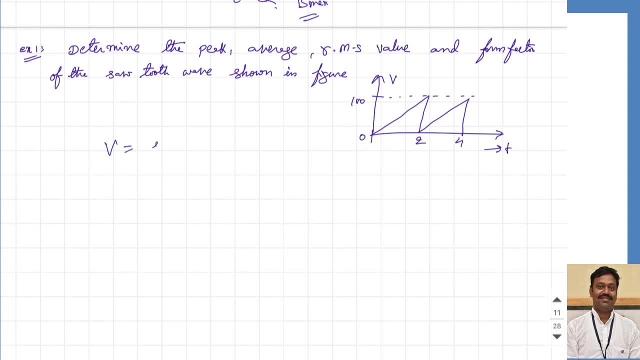 i can write equation for this one is equal to some slope. so what is the slope? multiplied by time, so it is having a slope. how to write the slope slope i can get by slope is equal to y 2 minus y 1, divided by x 2 minus x 1. what is the value of y 2? it is reaching up to 100 and y 1 is 0. 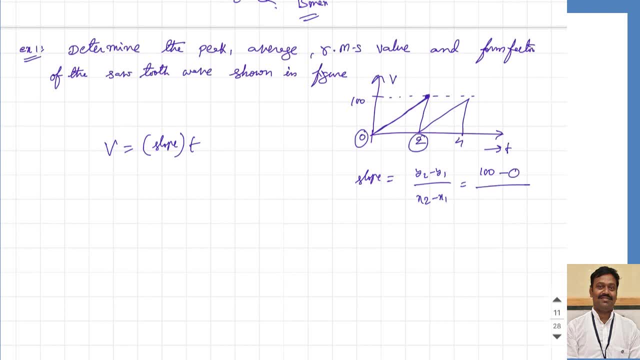 so 0 divided by x, 2 x 2 is it is going up to 2. so 2 minus 0. so this will become 50. that is my slope. that is my slope getting it. so in this example it is 50.. so if you write in a generalized way, so generalized wave, this will 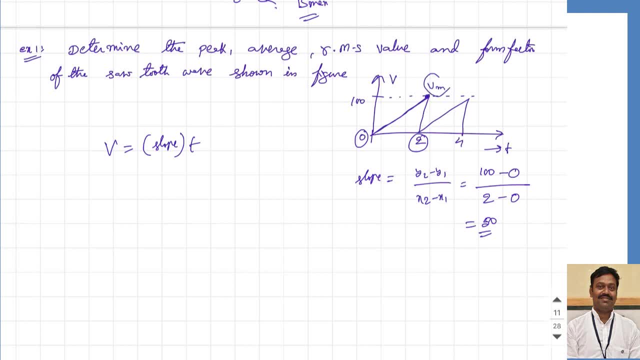 be equal to v maximum. let us take the maximum value as b maximum. so i'm just writing in a generalized way. then you substitute it so that it will become a generalized. so y 2 will become v max, become V maximum divided by 2.. So I can write: my instantaneous value of voltage is equal to. 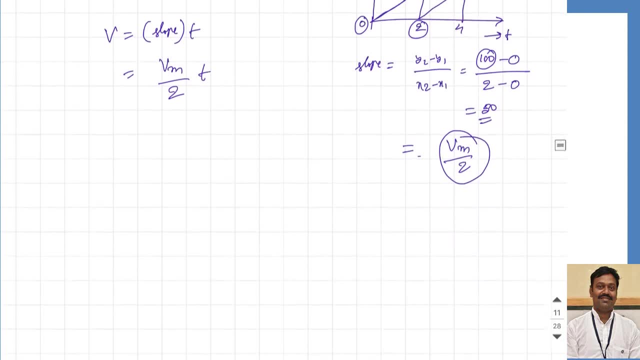 V maximum by 2 into T. Let us try to derive for this. So if you want to calculate the RMS value- so RMS value is root, mean, square value- So you have to take the root of square root of mean of the squares. So you have to take it 1 by 2 because time period is 2.. So 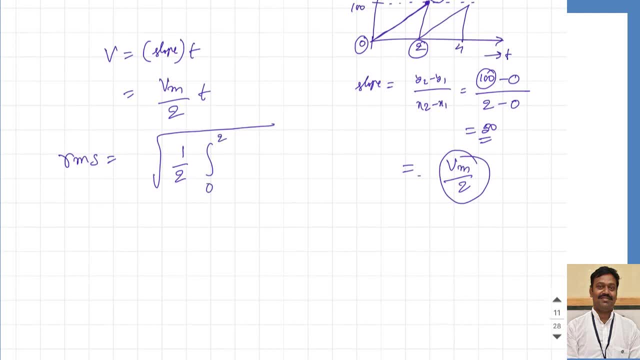 this becomes 1 by 2 integration from 0 to 2, because it is repeating from 0 to 2 every after 2 seconds. So this equation I got as V maximum by 2 into T dt. So I have to solve this So. 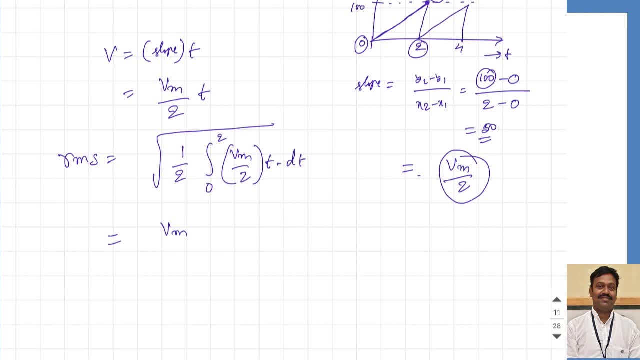 this I can write as this: V maximum. I can bring it outside. So you just I forget this V maximum by 2 into T. This equation I have to take square right. Root means square, So sorry, So this. 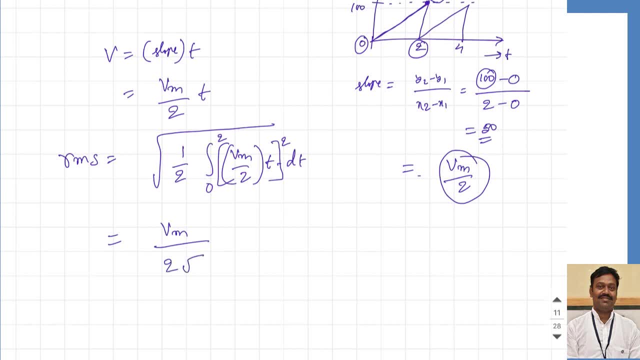 will come out. So this will come out as V maximum by 2 root 2.. Will come out square root of integration from 0 to 2.. This becomes T square dt. So if you substitute, you will get this as V maximum by root 3.. You will get this as V maximum by root 3.. So 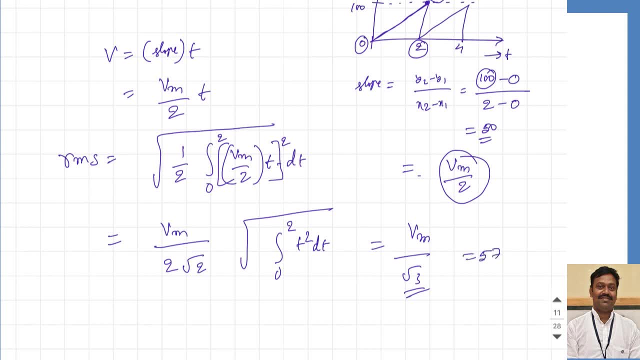 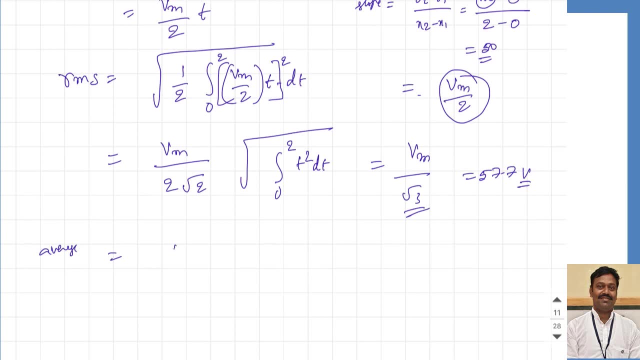 we know the maximum value in our example is 100.. If you substitute this, you will get it as 57.7 volts. Let us see how to calculate the average value. So average value will be equal to 1 by 2.. 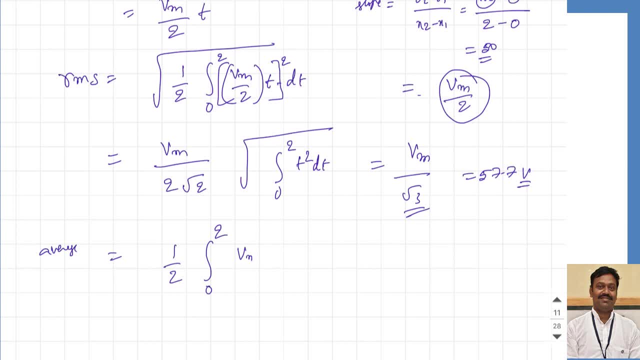 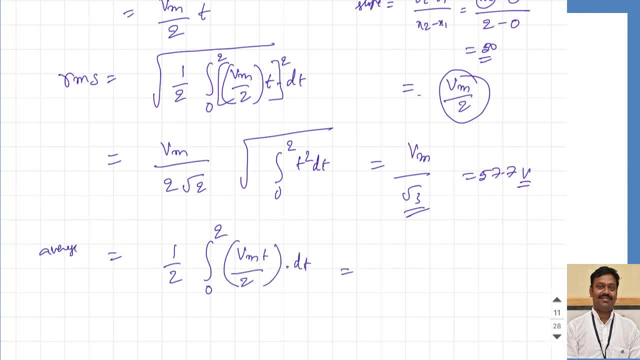 V maximum by 2 into T into dt. So again same thing. This V maximum by 4 will come out. So you have to take the integration from 0 to 2. T into dt. T become T square by 2.. So if you 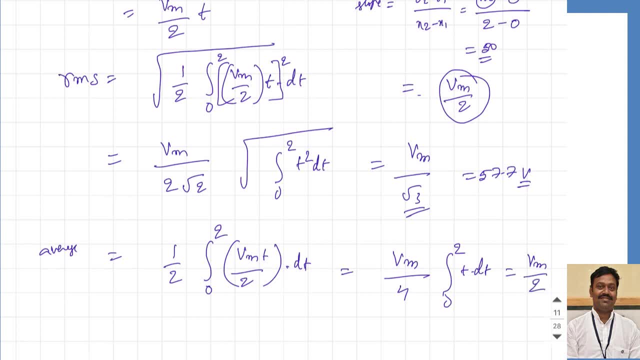 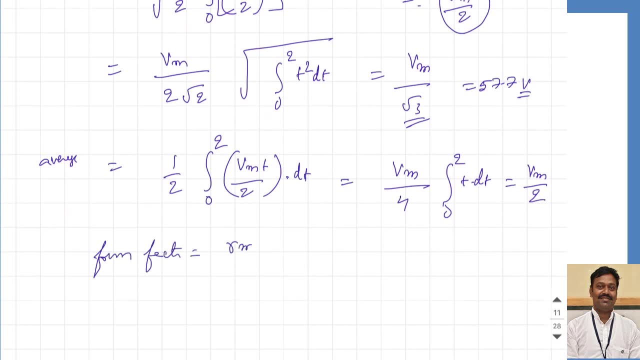 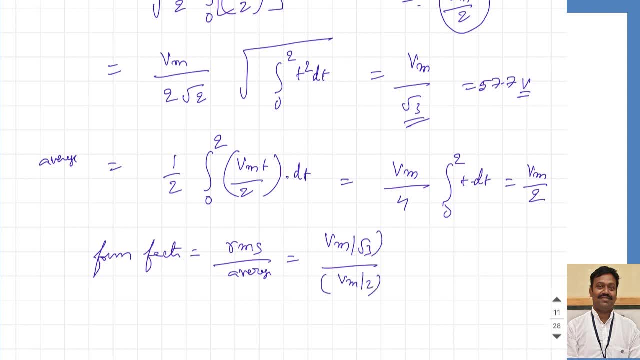 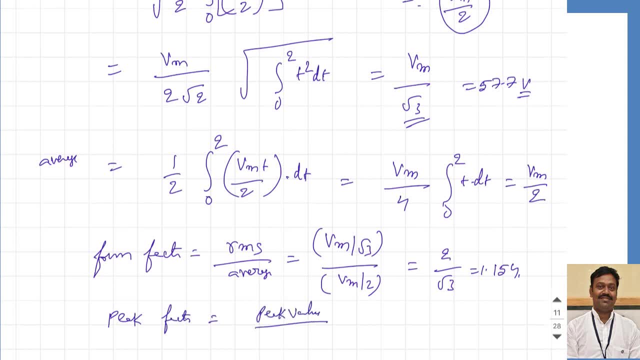 peak factor will be equal to the peak value divided by RMS value. So what is the peak value in this case? Peak value is 100.. RMS value is 57.7.. This will become 1.732.. You can see the. 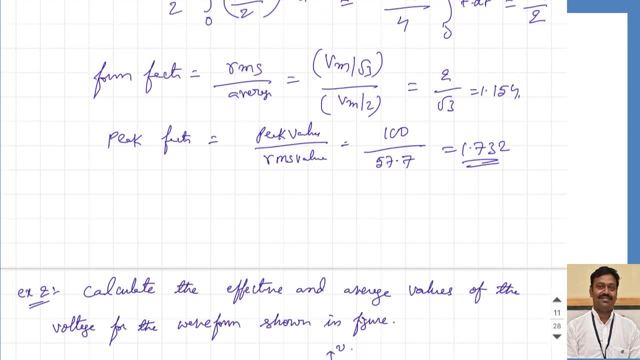 form factor is 1.732.. So you can see the form factor is 1.732.. So you can see the form factor and peak factor as different for the signal when compared to the sinusoidal signal. So let us take 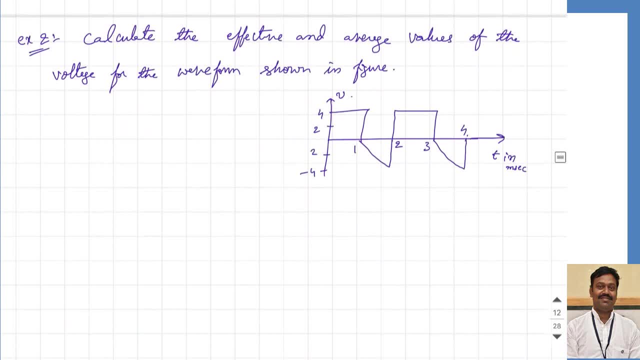 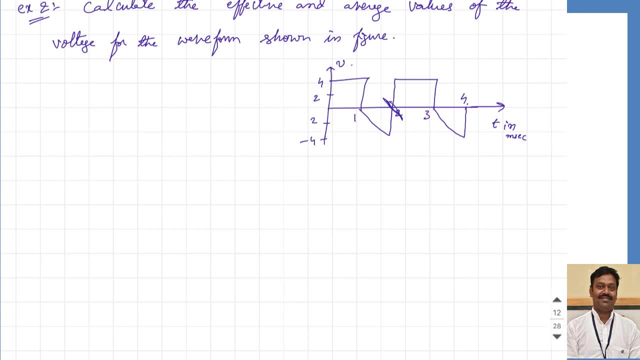 another example. So calculate the effective and average values for the signal shown in the figure. You can see this signal, It is not a symmetrical signal. It is varying after every 2 seconds. So I have to take from 0 to 2.. So out of 0 to 2, it is having 2 components. From 0 to 1, it is. 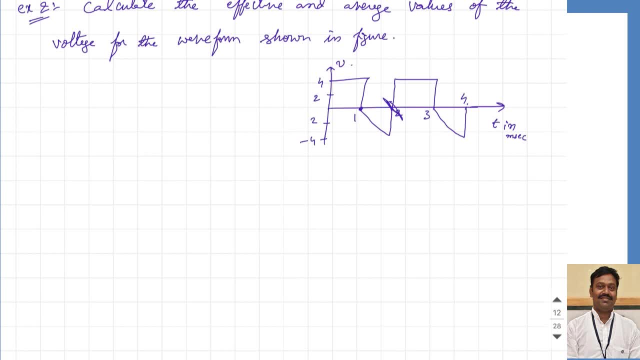 constant. After that it is having a slope. So how to write this slope? So again, to calculate this: if you have a slope, you have to write a slope. So again to calculate this: if you have a slope you have to write a slope. So if you have a slope, you have to write a slope. So 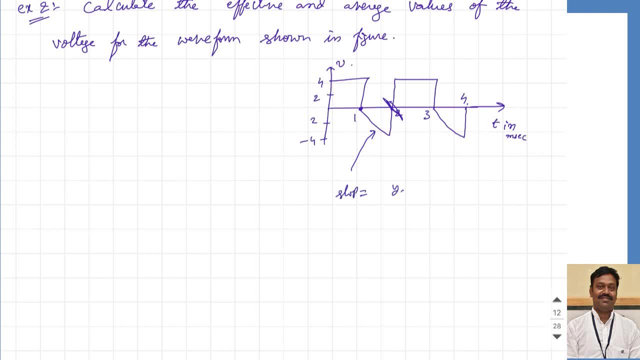 if you want to write the equation, so slope will be equal to y2 minus y1 by x2 minus x1. So y2, y2 means it is reaching from minus 4.. Minus 4, minus what is y1?? Because it is y1 is 0, y2 is. 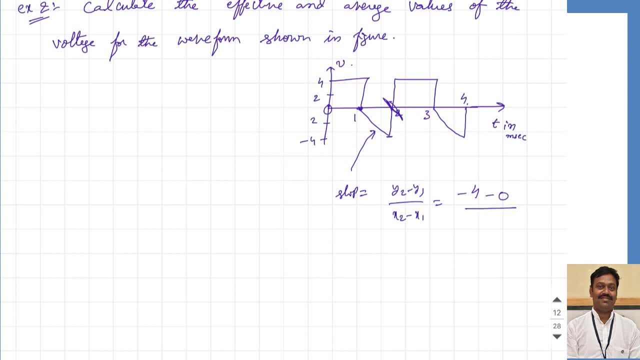 minus 4.. This is 0 divided by x2 minus x1.. x2 is 2 and x1 is 1, because this is from 1 to 2, 2 minus 1.. So this becomes 4 divided by 1.. So 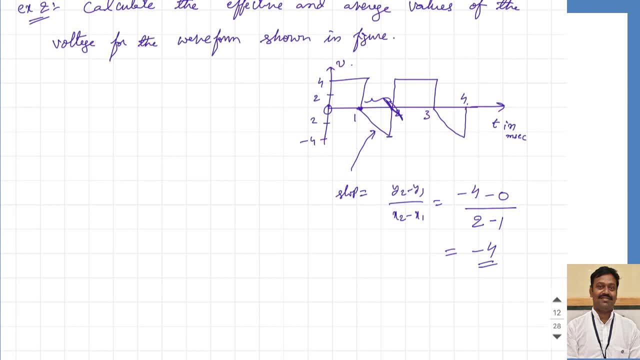 this becomes minus 4.. So slope, I got as minus 4.. So if you want to write the equation for this, you can write the equation by y minus y1, by x minus x1 is equal to y2 minus y1, by x2 minus x1. 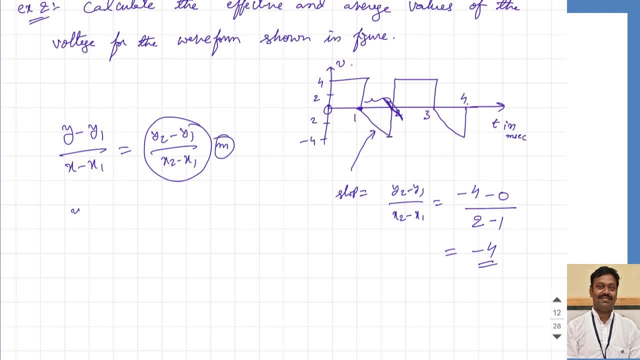 So this is nothing but the slope m. So I can write y minus what is the value of y1? for this curve, y1 is 0.. So y minus 0, divided by x minus what is x1?? x1 is in the 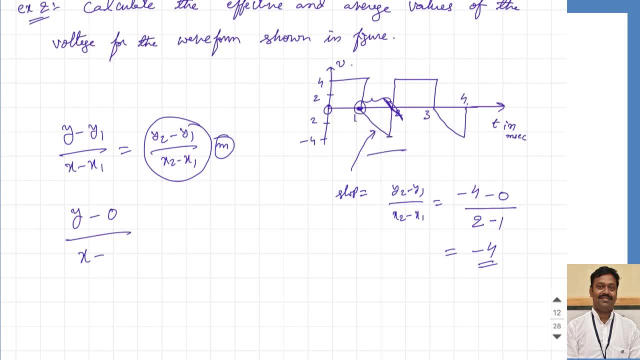 x axis. In this x axis this is equal to 1.. So I have to write: x minus 1 is equal to slope is minus 4.. Or from this I can write: y is equal to minus 4 into x minus 1.. Or this I can write as: 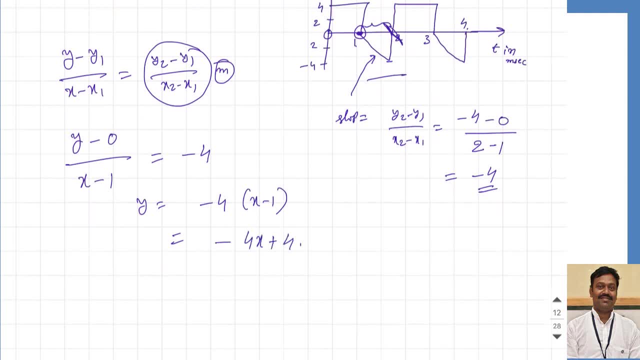 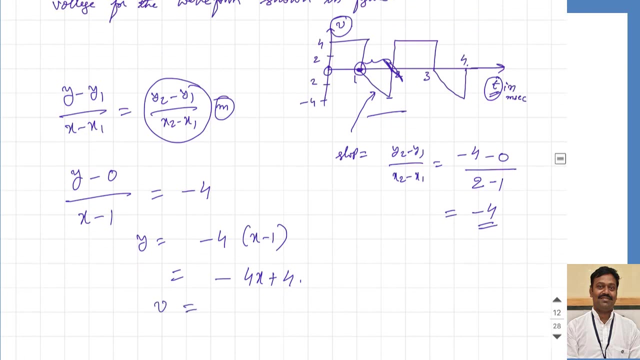 minus 4x plus 4.. Everyone agree with me: Minus 4 into x plus 4.. So what is x in our example? In our example, x is time And what is y? y is nothing but the voltage. So I am replacing that here. So this y is nothing but voltage is equal to. 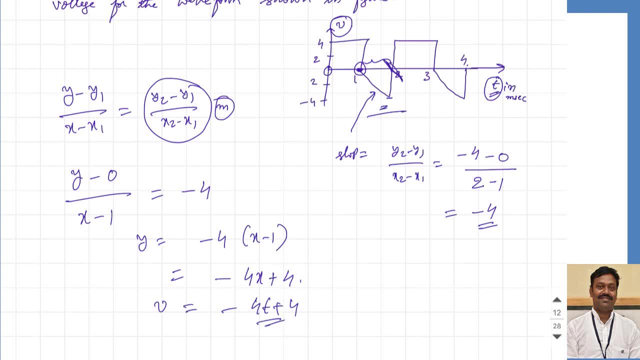 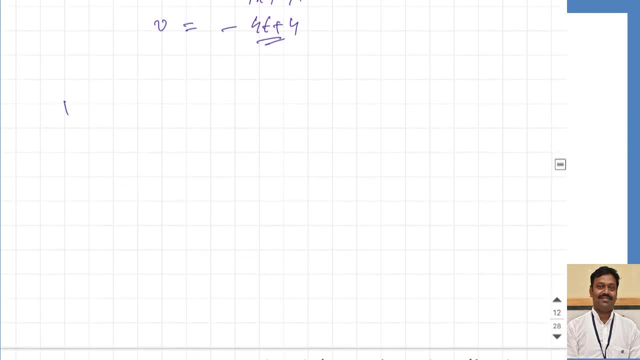 minus 4t plus 4 for this duration. For remaining, it is a rectangular wave, it will be constant. So with this O6, let us try to solve this- So I can calculate my value of V effective value or V rms value is equal to square root of, So total time period is 2,. 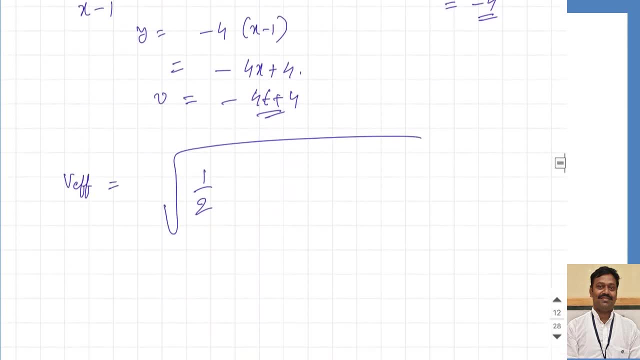 because it is varying from up to 2 seconds, So 0 to 2.. So that is why 1 by 2.. And this integration will have a value of 0. So that is why 1 by 2.. So that is why 1 by 2.. 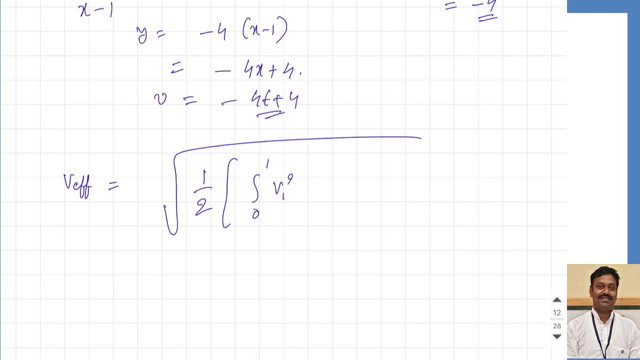 So I have two parts. 1 is 0 to 1.. 0 to 1, I have to take- let us assume voltage is V1, V1 square dt. Similarly, I have to take from 1 to 2, V2 square into dt. We will substitute these. 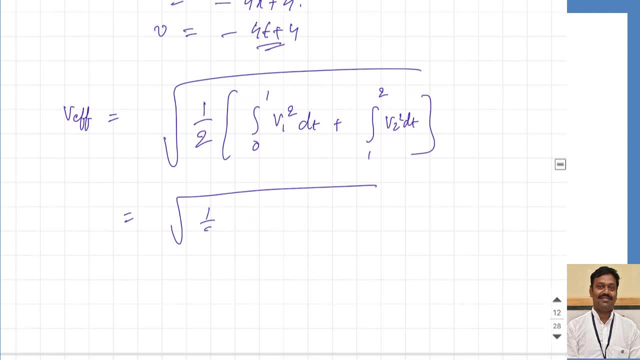 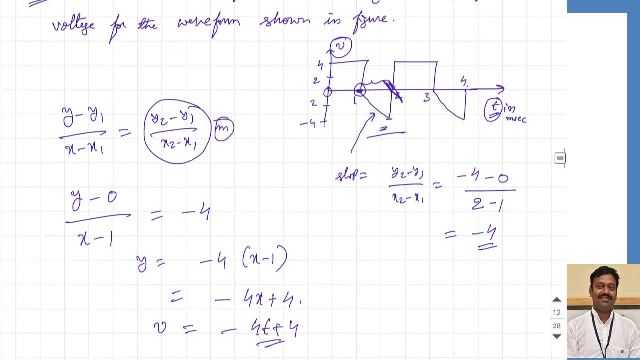 terms. So this I can write as square root of 1 by 2, integration from 0 to 1.. So from 0 to 1, the value is constant, And what is the magnitude? That magnitude is equal to 4.. So I am just. 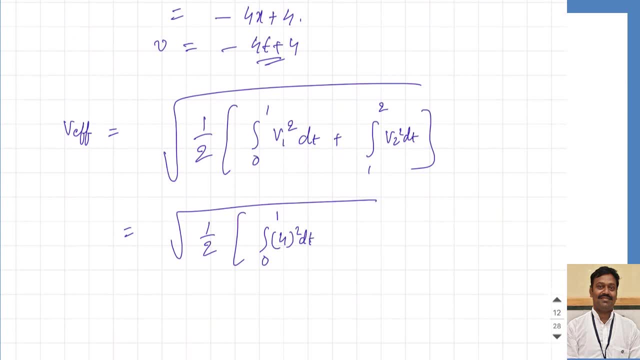 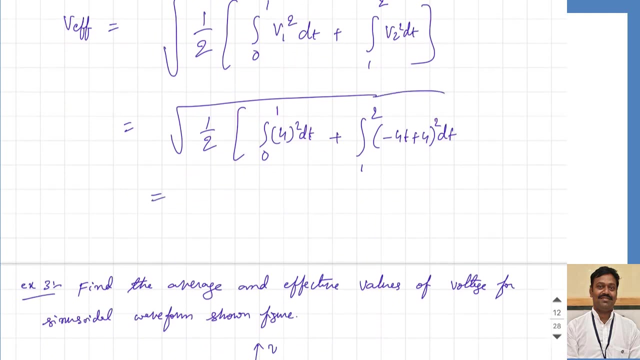 substituting that, This becomes 4 square. So this is the equation I get, So you can just expand them and solve it. I am directly writing the answer to save the time. So this you will get as 32 by 3 volts square root of. 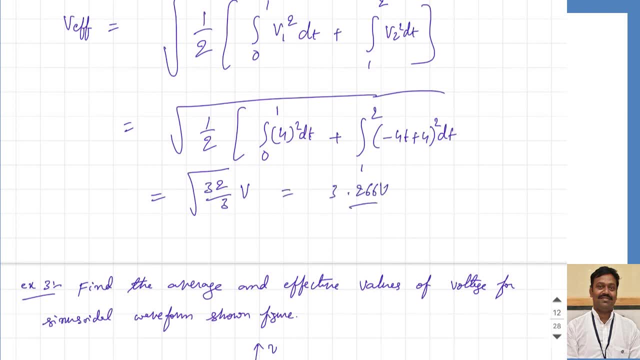 So this will become equal to 3.266 volts. This is my rms value. Similarly, if you want to calculate the average value, the average value will be equal to integration from 0 to 1, V1, dt or V1 is nothing but 4 dt. 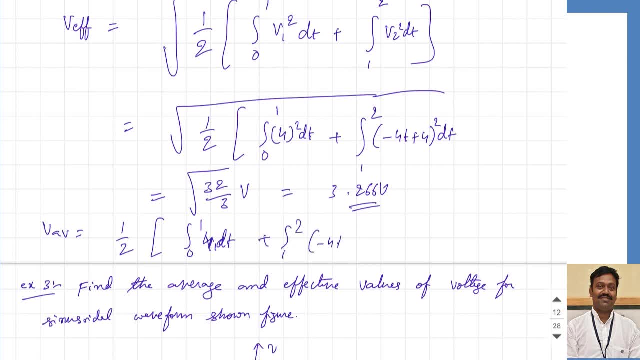 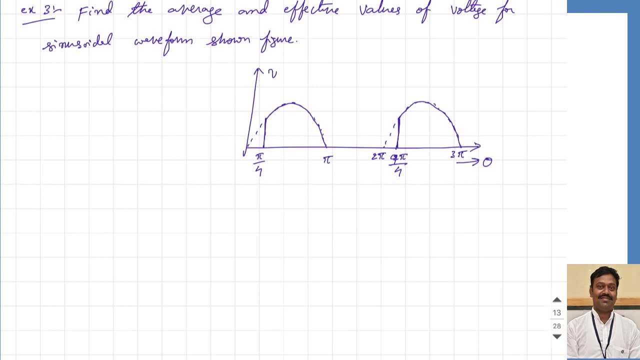 I am directly writing, plus integration from 1 to 2 minus 4, t plus 4 into dt. Just do the integration and substitute, You will get this as 1 volt. You can just cross verify your answer. So now I am taking another example. So this example: find the average and effective values. 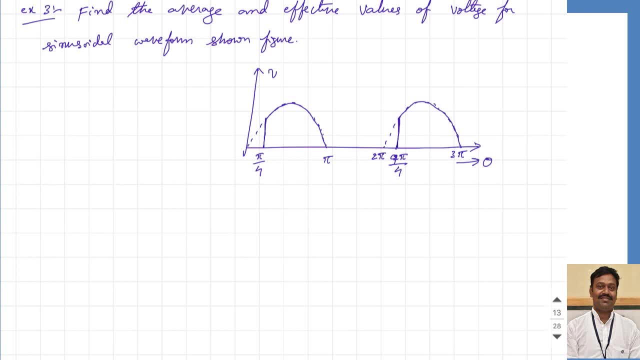 of the voltages for a sinusoidal waveform shown in figure. So the sinusoidal waveform is equal to the integral waveform of the sinusoidal waveform shown. So here. I forgot to mention, so have mentioned this as 100 volts. So this is the waveform given. So this waveform I. 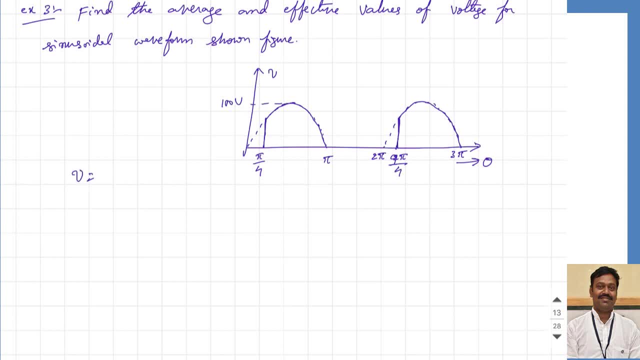 can write the equation. So I can write the equation for V. So V is nothing but V. maximum is 100 sine omega. t Out of this waveform is starting from here. This part is missing, that remaining part. So here we. similarly, this part is missing and waveform is symmetrical. up to 2pi. So we have to take the integration for entire 2pi. So we have to take the integration for entire 2pi. So here it is. So we have to take the integration for entire 2pi. So you. 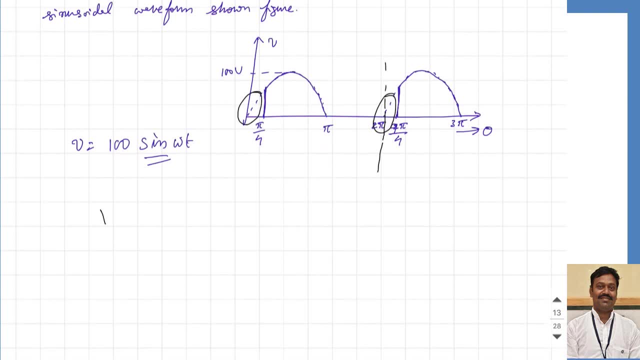 pi. that's why, to teach that one layer, i have taken this. so if i want to calculate the average value, v average value will be- you have to take for the entire duration. so 1 by time period is 0 to 2 pi and this waveform is varying from pi by 4 to pi. remaining is 0. so that's why i'm only taking from. 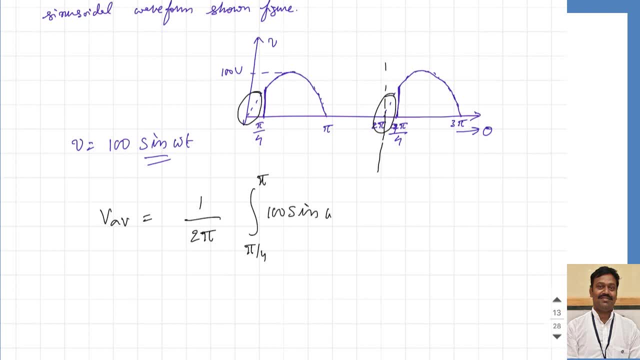 pi by 4 to pi: 100 sine omega t dt, 100 sine omega t dt or 100 sine theta d theta. i can write in a simple way, because all the omega and everything will go, so i'm just writing it here, sine theta d theta. i can write like this. so if you calculate this, so you are directly writing the answer. 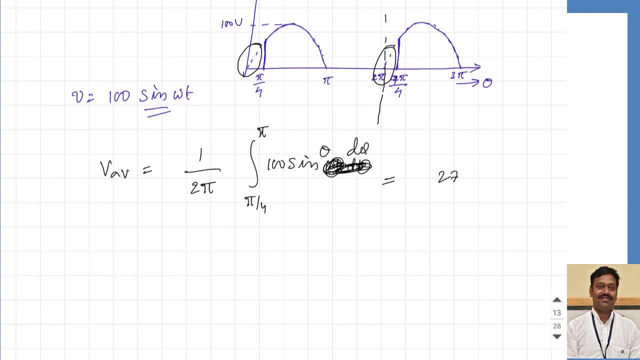 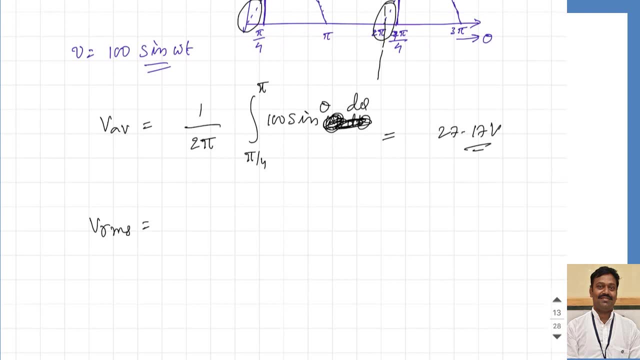 because the signs sine theta, that average value. if you substitute, you will get it as 27.17 volts you just cross. verify your result. so similar is the case v. rms value will be 1 by 2 pi, integration from pi by 4 to pi 100 square. 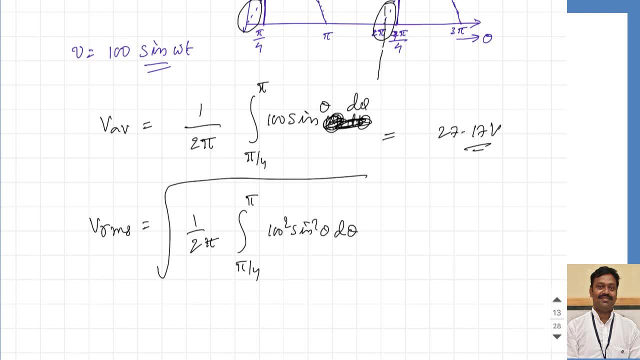 you can write like this: so if you calculate this, so you are directly writing the answer, because sine square theta, d theta, this entire thing, i have to take the square root again. same thing. if you solve it by taking 1 minus cos 2 theta and substituting and solving it, you will get this. 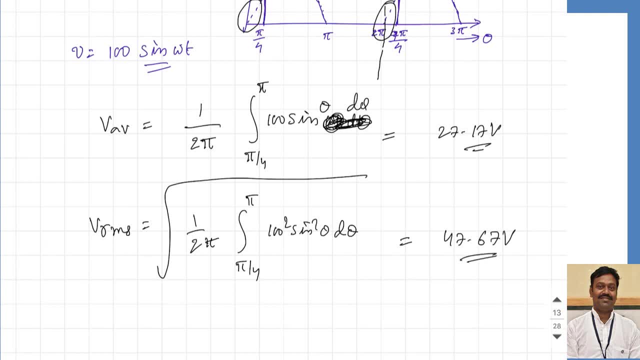 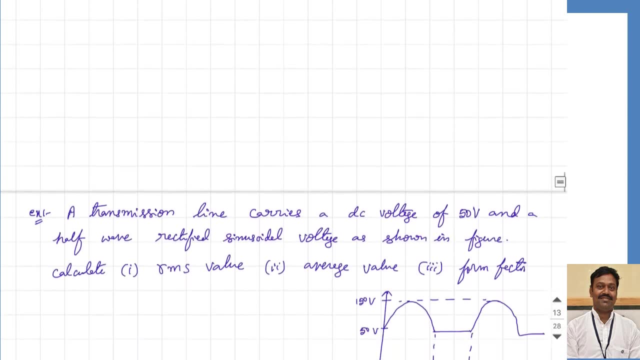 answer as 47.67 volts. i am directly writing the answer because i hope you have. you are good in the mathematics. you can solve it and cross verify. if you are not getting, you can leave your comments in the comment section. i will answer and provide you the things. so now i am taking one more example. 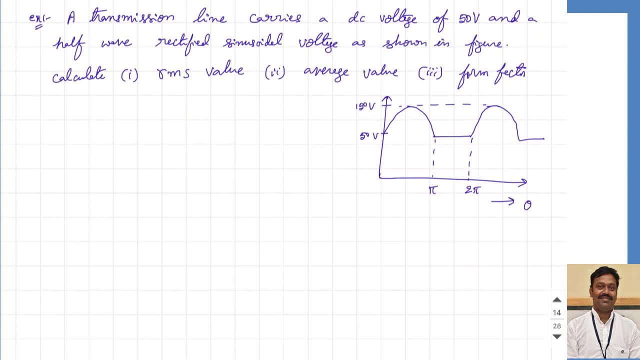 a transmission line carries a dc volt, voltage of 50 volts and a half-way rectifier sinusoidal voltage as shown in the figure. calculate the rms value, average value on the form factor. so you can see here it is having two signals. one signal is a dc, another signal is ac. so there are two things. one is 0 to pi and pi to 2, pi, pi to. 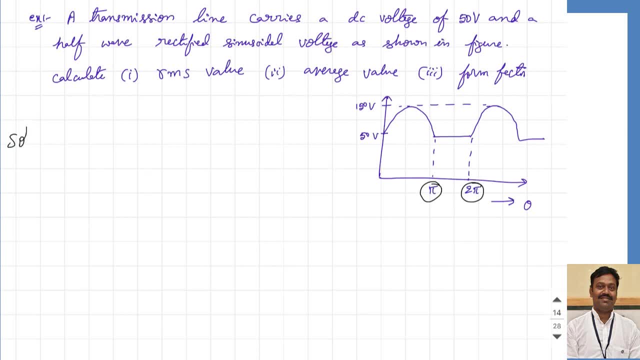 2 pi. it is not 0, it is having 50 volts. so i can divide this into two parts. one is v is equal to 50 plus, so what is the difference between the two parts? one is v is equal to 50 plus, so what is the? 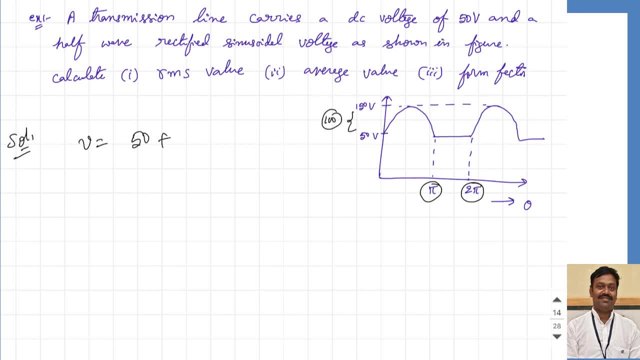 difference in magnitude between these two: 150 minus 50 is 100. that means maximum value of this sine wave is, if you are taking this as a sine wave, half a rectified sine wave magnitude is 100. so i can write it as v maximum into sine theta. this is for 0, less than theta, less than pi. so now v from.